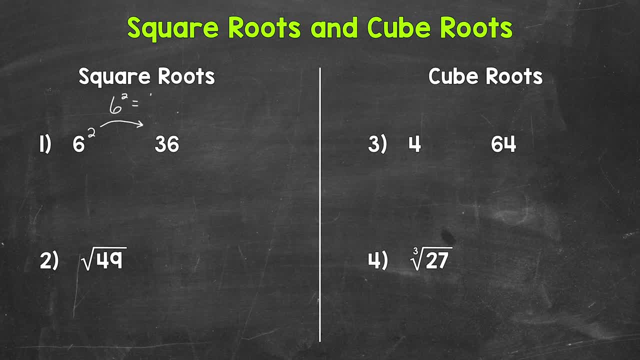 So 6 squared means 6 times 6., Which equals 36.. So again, 6 squared equals 36.. Now the square root of a number is the inverse, or opposite of squaring a number. We are going in reverse of squaring a number, so to speak. 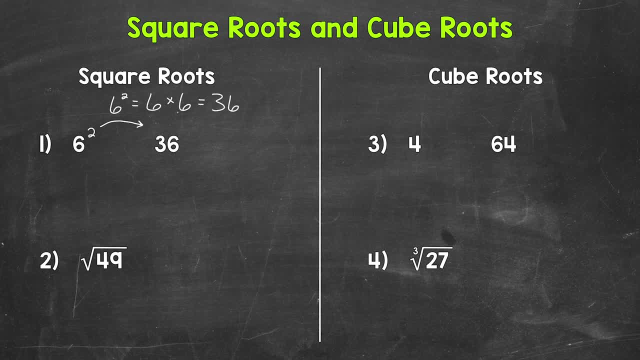 When it comes to square roots, we need to think what number multiplied by itself will equal the number under the root symbol. For example, let's find the square root of 36.. So what number multiplied by itself equals 36?? Well, we know that 6 times 6 equals 36.. 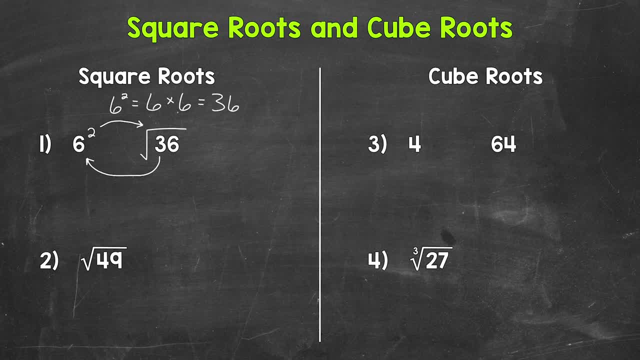 So the square root of 36 is 6.. Again, the square root of 36 equals 6.. Let's move on to number 2, where we have the square root of 49. Well, what number multiplied by itself equals 49?? 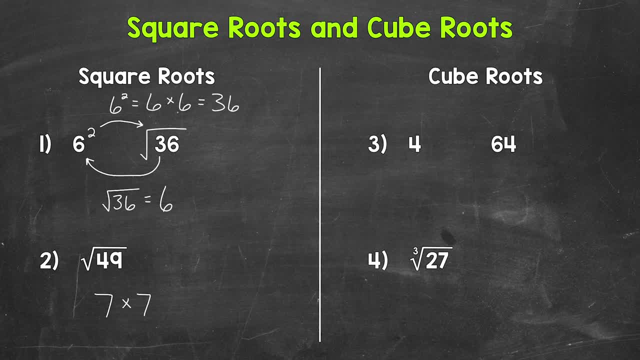 We know that the square root of 49 is 6.. So again we need to think what number multiplied by itself equals 36.. that 7 times 7 equals 49. That means that the square root of 49 equals 7.. So there's a brief. 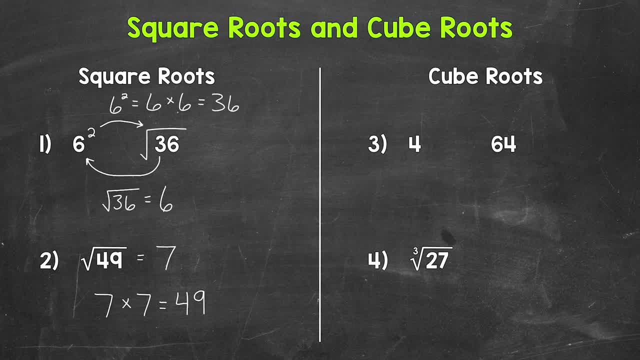 overview of square roots. Let's move on to cube roots and take a look at numbers 3 and 4.. Starting with number 3, where we have a 4 and a 64.. Now, in order to understand cube roots, we are going to 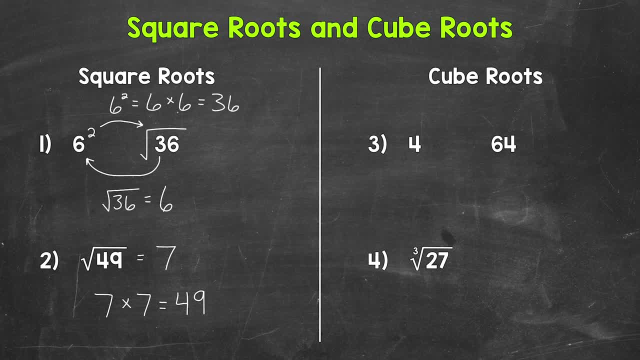 start by looking at cubing a number. For example, let's do 4 cubed Now. 4 cubed equals 64. When we cube a number, we multiply that number by itself three times. So 4 cubed means 4 times 4 times 4.. 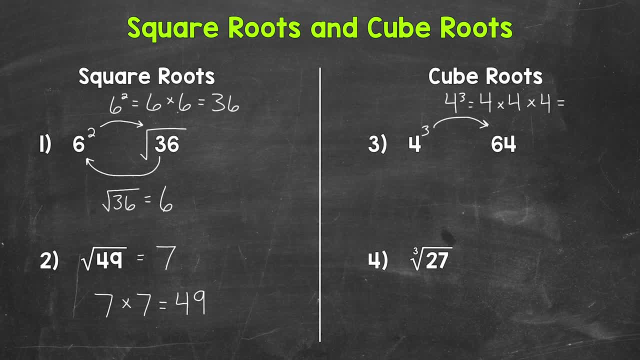 4 times 4 is 16 times 4 is 64. So again, 4 cubed equals 64. Now the cube root of a number is the inverse or opposite of cubing a number. We are going to go in reverse of cubing a number, so to speak. When it comes to a cube root, we need to think what. 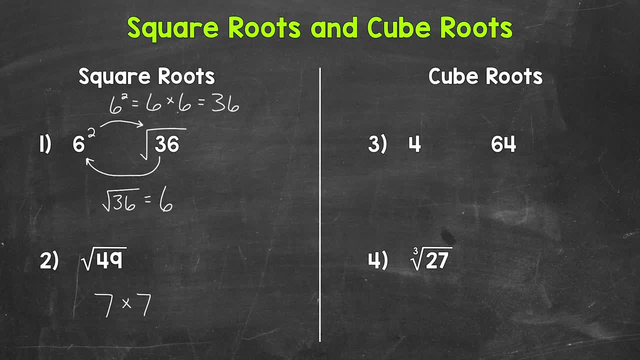 We know that 7 times 7 equals 49.. That means that the square root of 49 equals 7.. So there's a brief overview of square roots. Let's move on to cube roots and take a look at numbers 3 and 4.. Starting, 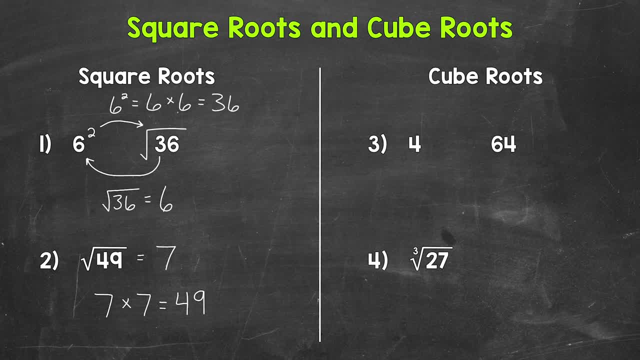 with number 3, where we have a 4 and a 64. Now, in order to understand cube roots, we are going to start by looking at cubing a number. For example, let's do 4 cubed. Now, 4 cubed equals 64. When we 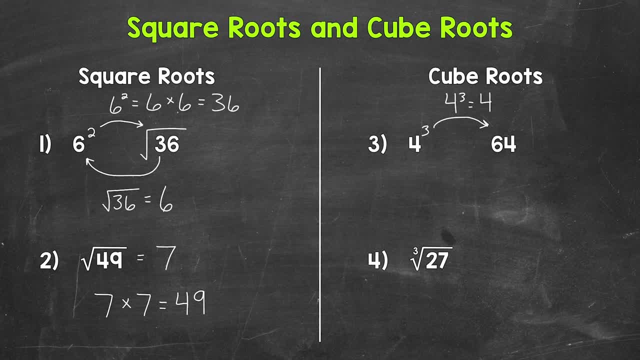 cube a number, we multiply that number by itself three times. So 4 cubed means 4 times 4 times 4.. 4 times 4 is 16 times 4 is 64. So again, 4 cubed equals 64.. Now the cube root of a number is the inverse or opposite of cubing a number. We are going to go. 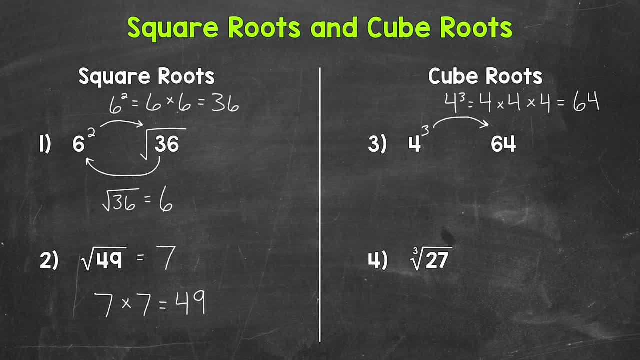 in reverse of cubing a number, so to speak. When it comes to a cube root, we need to think what number multiplied by itself, three times, equals the number under the cube root symbol. For example, 3 times equals 64. Well, we know that 4 times 4 times 4 equals 64. So the cube root of 64 is 4. Again. 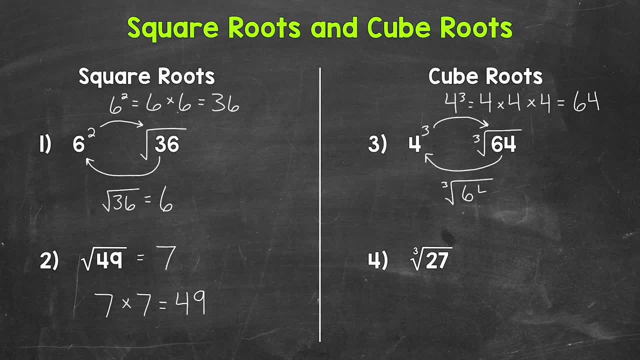 the cube root of 64 equals 4.. Let's move on to number 4, where we have the cube root of 27.. So what number, multiplied by itself, three times, equals 27?? Well, we know that 4 times 4 times 4 equals 64. So 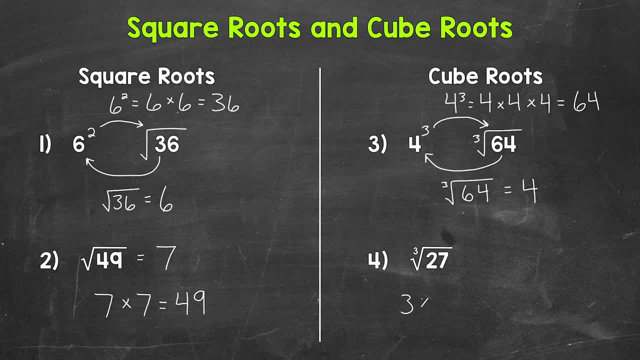 what number multiplied by itself three times equals 27?? Well, 3 times 3 times 3 equals 27.. 3 times 3 is 9 times 3 equals 27.. That means that the cube root of 27 equals 3.. So there's a brief overview of. 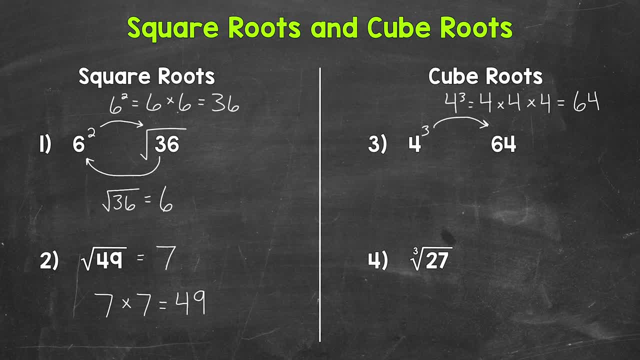 number multiplied by itself three times equals the number under the cube root symbol. For example, 3 times equals 64. Well, we know that 4 times 4 times 4 equals 64. So the cube root of 64 is 4. Again. 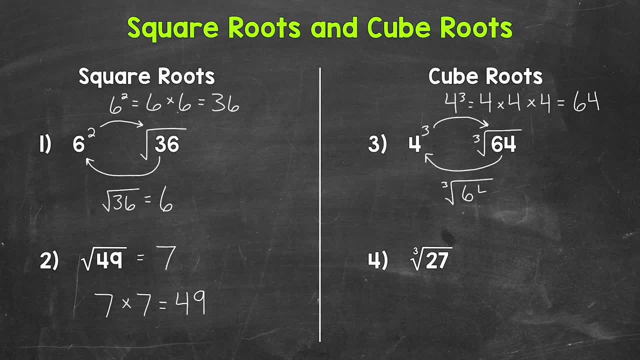 the cube root of 64 equals 4.. Let's move on to number 4, where we have the cube root of 27.. So what number, multiplied by itself, three times, equals 27?? Well, we know that 4 times 4 times 4 equals 64. So 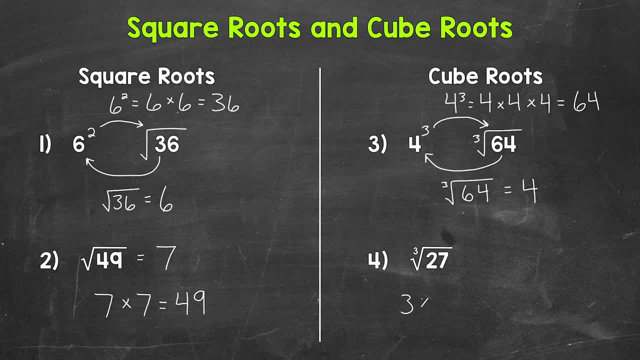 what number multiplied by itself three times equals 27?? Well, 3 times 3 times 3 equals 27.. 3 times 3 is 9 times 3 equals 27.. That means that the cube root of 27 equals 3.. So there's a brief overview of. 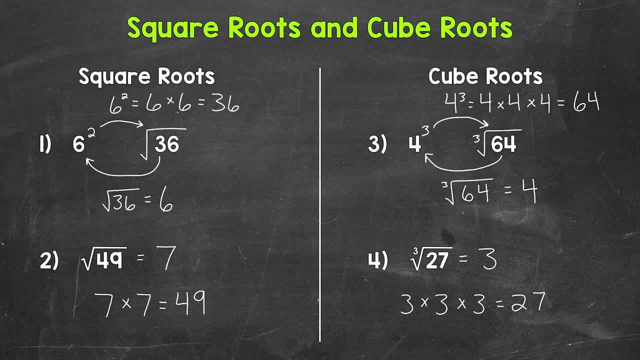 cube roots. Now to recap. for square roots, we need to think about what number multiplied by itself will equal the number multiplied by itself. So we're going to go in reverse of cubing a number under the root symbol. For cube roots, we need to think about what number multiplied by itself 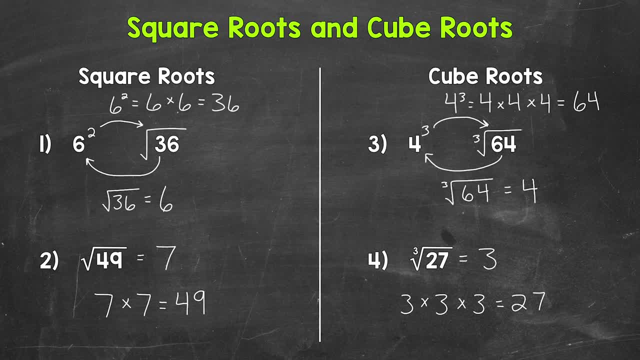 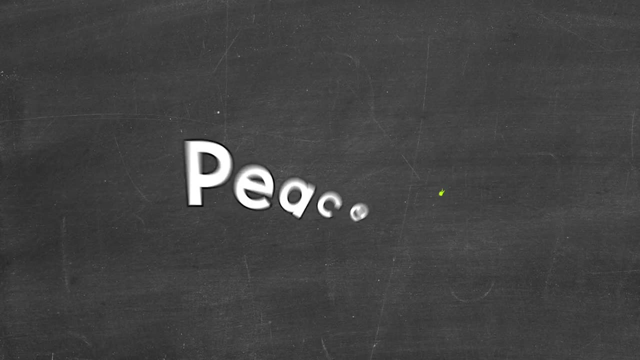 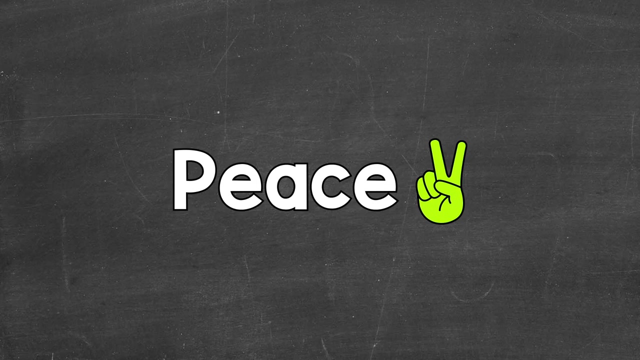 three times will equal the number under the cube root symbol. So there you have it. There's an explanation of square roots and cube roots. I hope that helped. Thanks so much for watching. Until next time, peace. Captions by GetTranscribedcom.